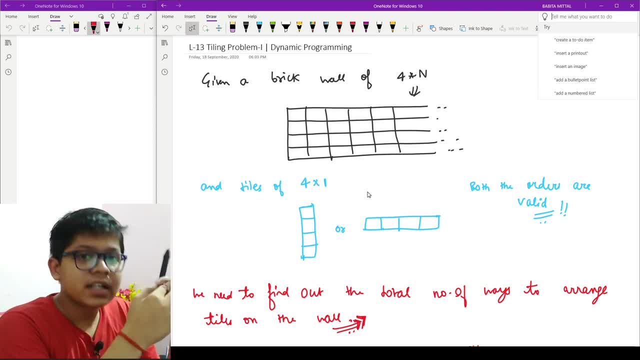 total number of ways to arrange this tile on the grid wall right, so like: if you go on approaching this problem, so the first thing if you go on approaching this problem, so the first thing. if you go on approaching this problem, so the first thing if you go on approaching this problem, so. 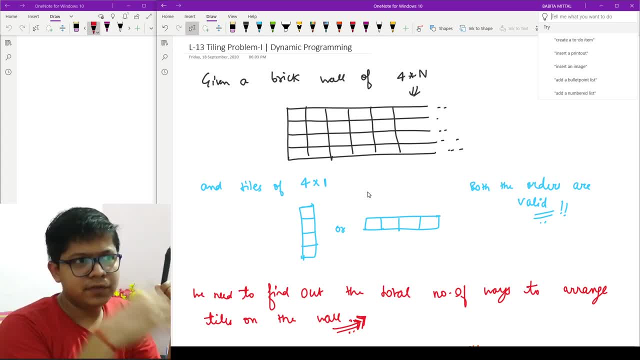 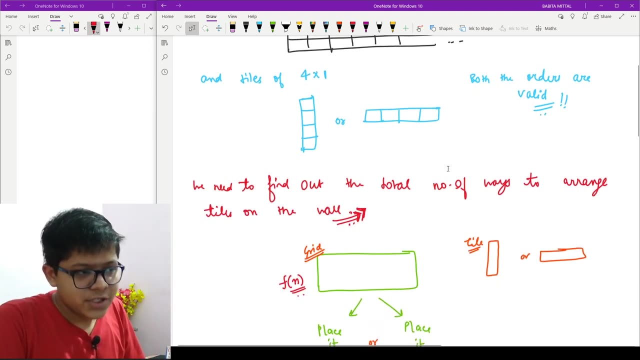 you want to place this on your grid wall. so the first thing you will think: okay, either i should place it vertically or i should place it horizontally. okay, so if like, if you place it vertically, then what will happen, and if you place it horizontally, then what will happen? so, before going on to what, 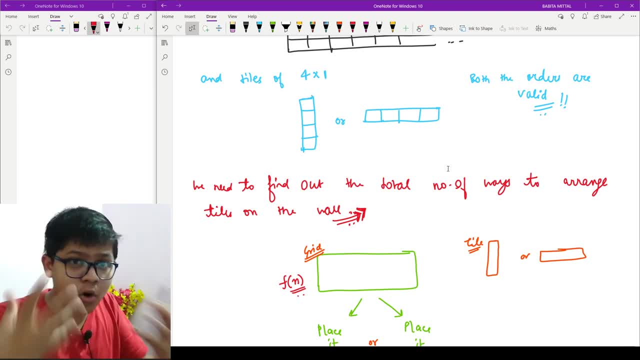 will happen. the first thing which you spoke was: either i can place it vertically or i can place it horizontally. so my emphasis on or was that i will find out the ways of placing it vertically, that if i place it vertically. so what are the number of ways i can obtain? and i will add those. 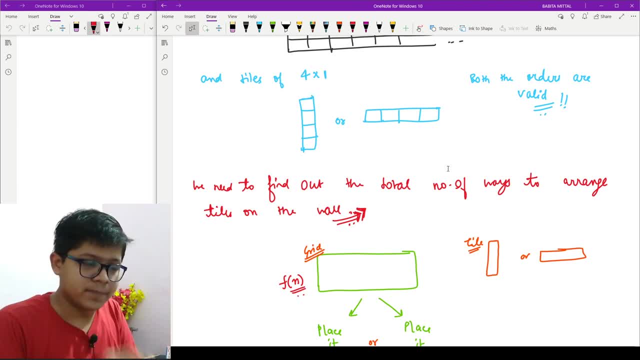 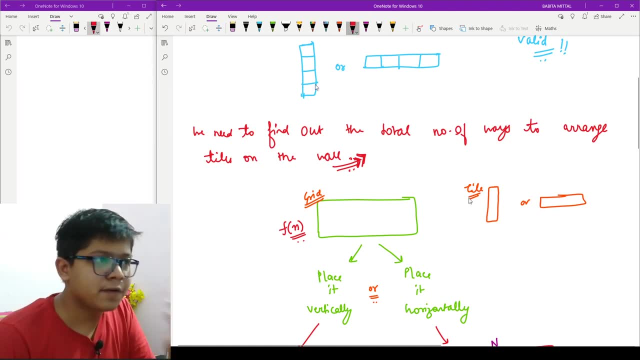 ways, with the ways i will obtain by placing it horizontally. now let's see with the figure that if i have this grid right here and if i represent my variable as f of n, that okay, f of n indicates the number of ways of placing my tile on this grid. so yeah, now the first option is i can place it vertically. so if i place it, 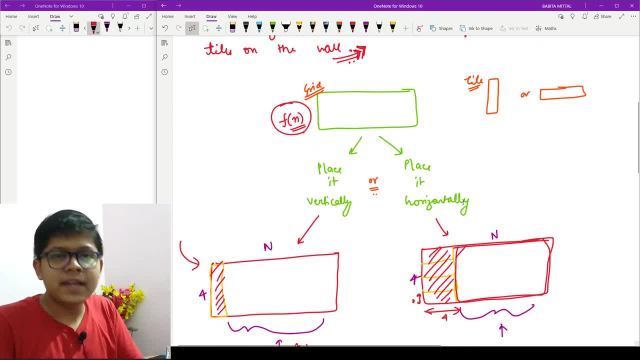 vertically. so what will happen is that it will occupy one column and four rows, as you can see here. now the problem is reduced to a problem that i need to find out my number of ways of placing my tile on this n minus one column grid so i can place it vertically. so if i place it vertically, 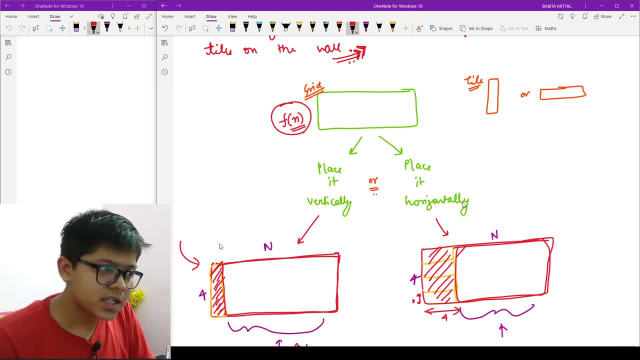 then what will happen is that it will occupy one column and four rows, as you can see the number of ways of placing my tile on this grid, which means that four rows and ms1 columns. so if anyhow i can find the answer for this, which is f of n minus one, because, as you can see, that one column is. 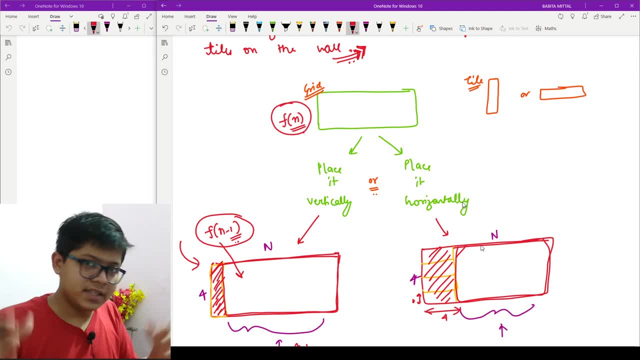 removed now. okay, like i, i will have this answer with me. uh, if anyhow i can find the answer for the other one, then i will add those answer. to obtain the answer for f of n now, the another option was i can place it horizontally. so if i place my horizontally, then see now if i place it. 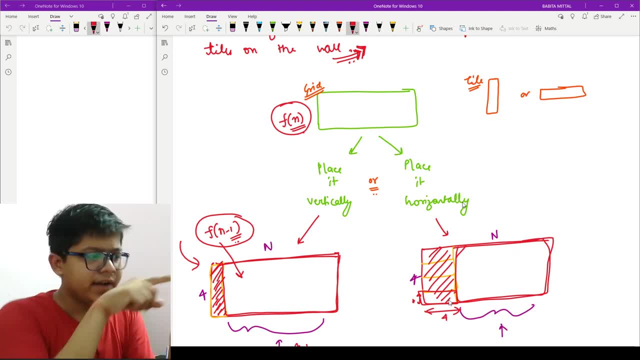 horizontally. after that you will, you can say that okay, and why not? you place another one vertically above it. so see, if i place it horizontally, then, uh, my number of rows remaining are three right, and to place another one above it vertically, i need four rows right, but it is only having three, so 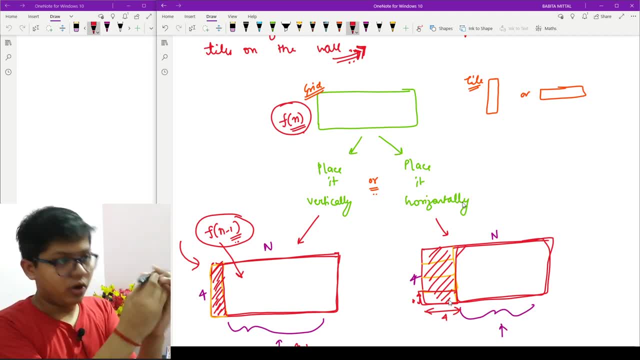 to place, like if i place my one horizontally, so i have to place other three also horizontally. thus, my sequence will look something like this: like horizontal here, horizontal here. all right, now the problem is reduced to a problem, that it is this, which means that, as you can see, 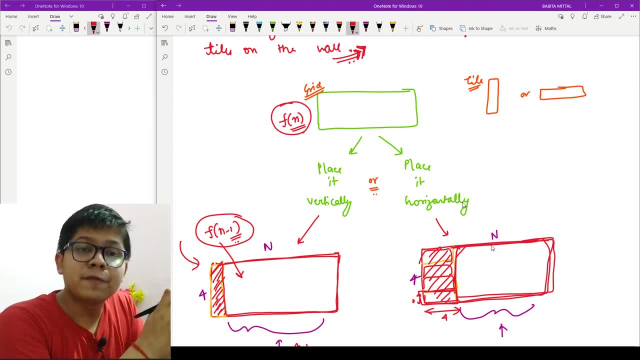 that my four columns are utilized and remaining columns are n minus 4.. so my problem is reduced to a problem of f of n minus 4.. now, as i said that, either i can place it vertically or i can place it horizontally. so if i place it vertically and horizontally, and i i have those ways in f of n minus. 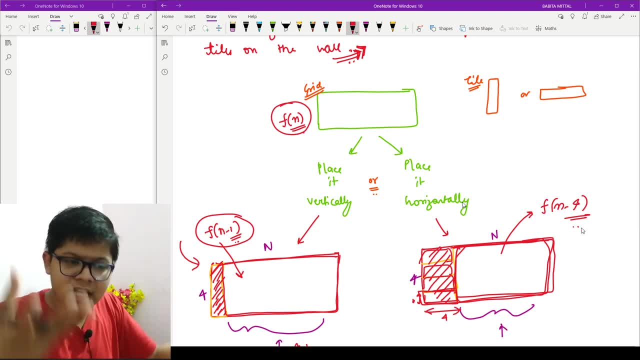 4, then I can add those ways, because I place my all sign here right, so I can add those ways to obtain the answer for f of n. so now you have reached your recurrence relation, which is f of n equal to f of n minus 1 plus f of n minus 4. very fine, now, as you can see here, I also showed that. 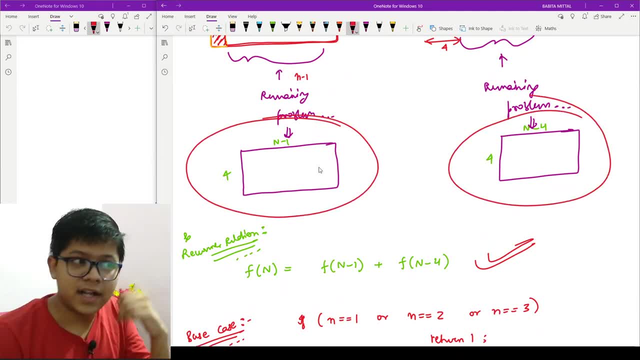 the remaining column is like this, and the remaining column for this is like this, and for those I have found out my recurrence relation and I added those to obtain my recurrence relation. finally, now comes the base case part. I have always said to you that think of the base case like okay. 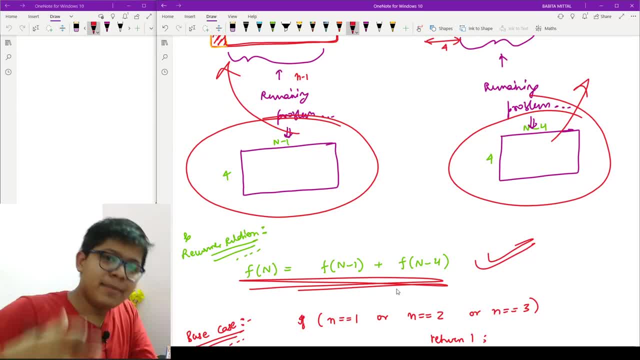 at what valid value of n. I would be easily able to find my answer, which means that think that if I place my 1 as the n, like say, you need to think that, okay, if I run the loop, then at what stage? like the, uh, the stage at which it. 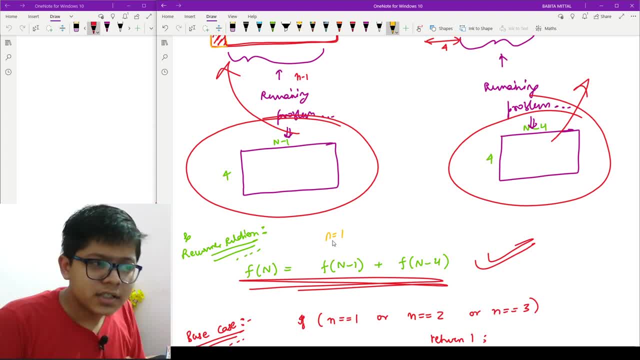 like it will, uh, not verify. I should say the answer, which means that if I place 1, so my f of it will go to minus 3. so, yeah, I cannot place it as a main case, so I need to place it as a base case. okay, my n equal to 2. then if I place it, so it will go minus 2, which is also not good. so I'll. 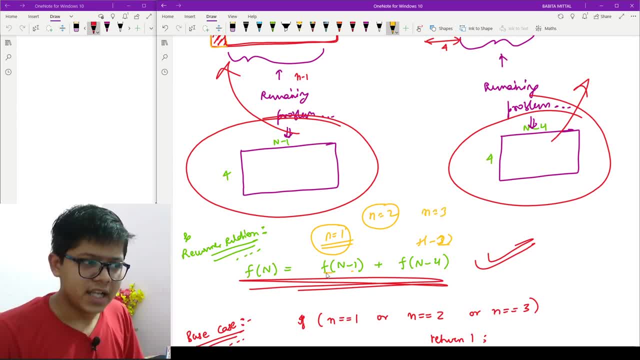 place it as a base case n equal to 3, then I will place it. okay, it is fine, but it will go to minus 1, which is also not good. so it is also a base case n equal to 4, then it will be something good. it will be f of 0, so either I. 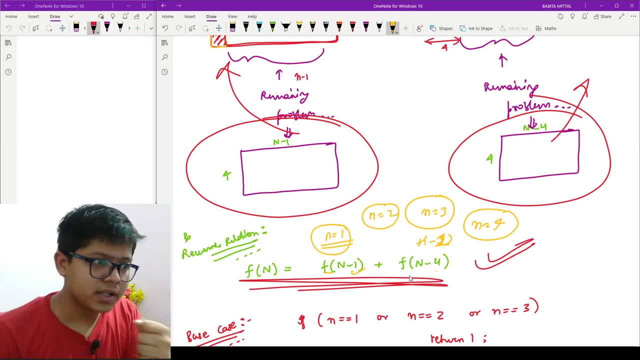 can place f of 0 as a base case, or I can place n equal to 4 as a base case, but if I place n equal to 0 as a base case, then I clearly know that my grade will be like something right. it will not be. 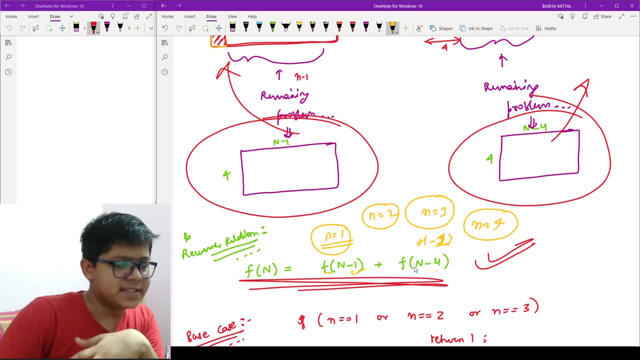 of n equal to 0. so I will place my n equal to 4 as a base case, rather n equal to 0 as a base case, although you can have 0 as well, but it is basically preferred to have a valid base cases which can be included in your answer as well. so, yeah, these would be your base. 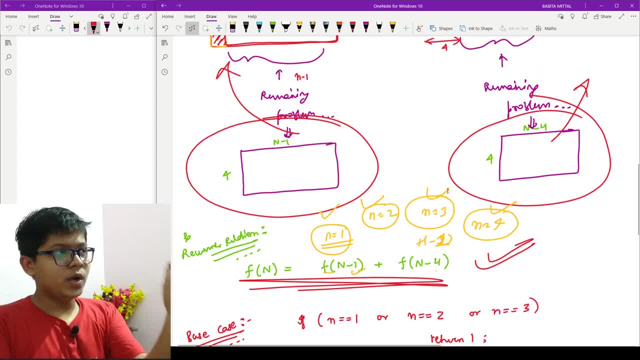 cases. now, as you can see that for n equal to 1 you have n equal to 1, which means that you have only this. so you can only place one tile here. so it's a one way. if n equal to 2, then also you can. 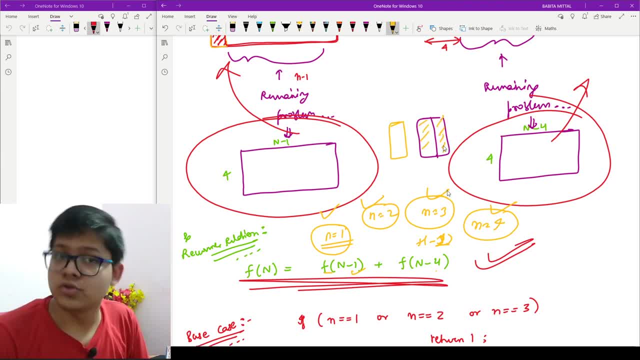 place vertically, vertically only, so it's also a one way. for n equal to 3, 1, 2, 3, you can also place vertically, vertically, so it's also a one way. so, as you can see that for n equal to 1, 2 or 3, my 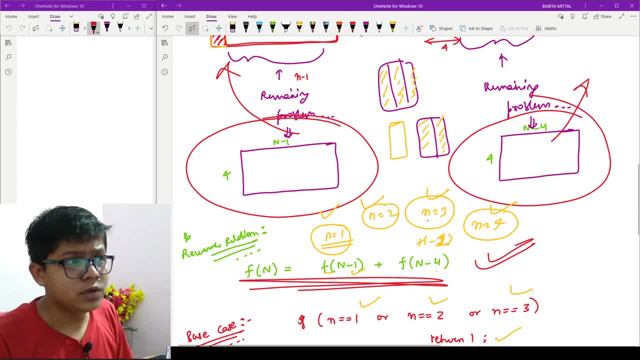 return case would be 1. only now you might think that for n equal to 4, what will happen for n equal to 4? see n equal to 4. so as I showed you that I can place it horizontally, so if I place it horizontally so I have to place all other horizontally as well. so it's a one way, or? 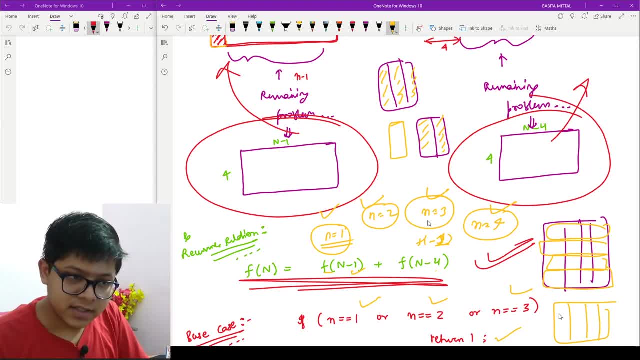 if I place it vertically, 1, 2, 3, 4, yeah, so I need to place my others vertically as well, because it needs at least four cells to place. so for n equal to 4, either I can place all horizontally or all vertically, so it's a two-way. so these would be the base cases and these it's a. 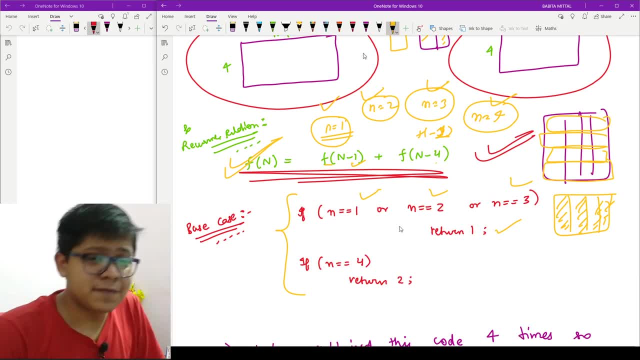 reconciliation. so like it's exactly same as Fibonacci series I taught you in the lecture 3 or 2, I guess. so I hope that by now you should be able to write its code and the efficient ones as well, because, like I said, I don't know how to write it, but I hope that by now you should be. 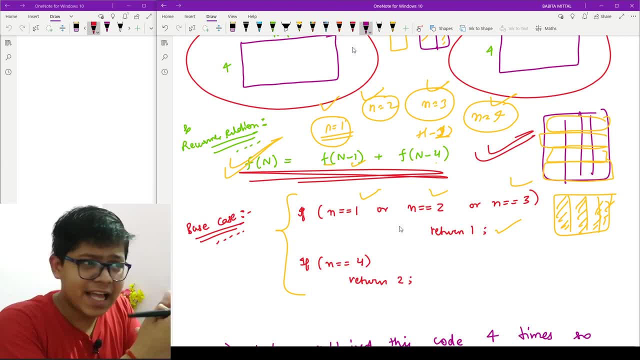 able to write its code, and the efficient ones as well, because, like I said, I don't know how to write. it has been for, I guess, 4 videos that I have been teaching the problems related to it. the main part is not to write the code after this, because after this that you have written the code many times. but